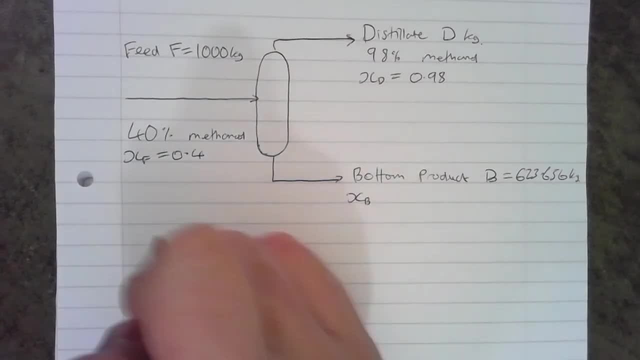 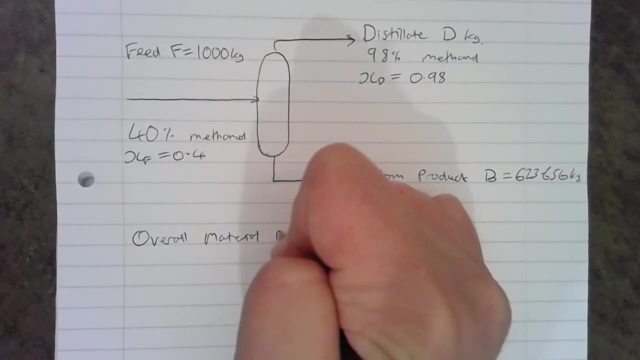 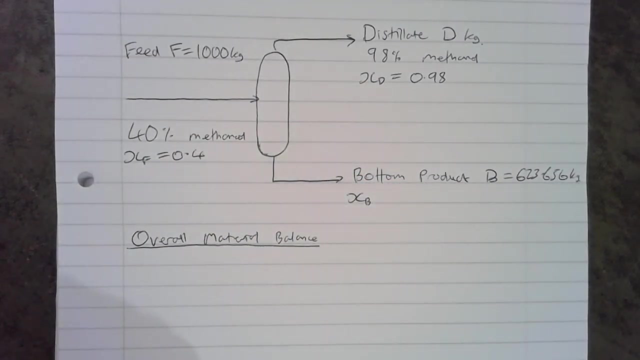 Now that we've done the diagram, we need to do an overall material balance. Now we know what goes in, must come out, because we've got a steady state operation, steady state process with no reaction, and so the feed equals the distillate plus the bottom product. 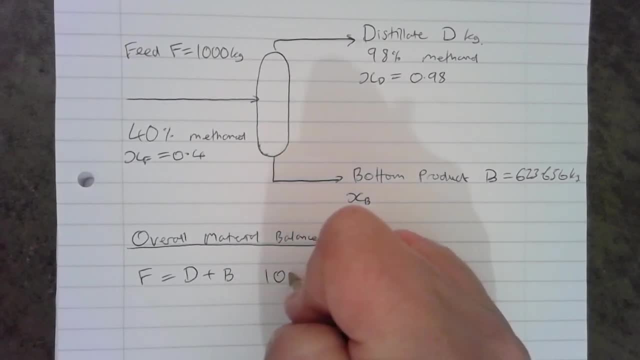 And we know actually that the feed is 1000.. 1000 equals- we don't know the distillate- that's D plus 623.656 grams of ethanol. that's D plus 623.656 kilograms of ethanol. That's D plus 4.5 kilograms of ethanol. That's D plus 4.5 kilograms of ethanol. 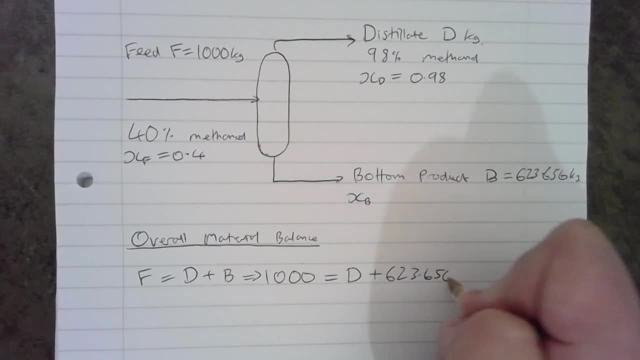 And we know that the step is one. we've got to do one step at a time because we know what goes in must come out. We can rearrange that: D equals 1000 minus 623.656 equals 376.344 kilograms. 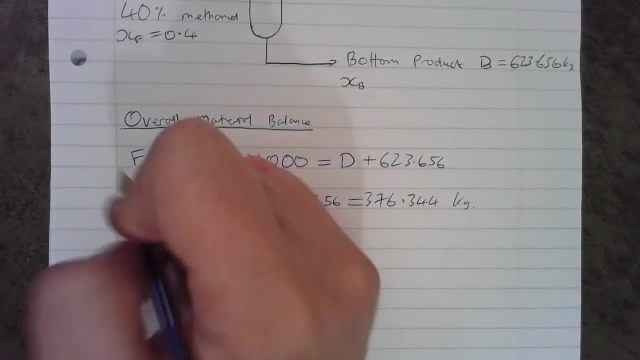 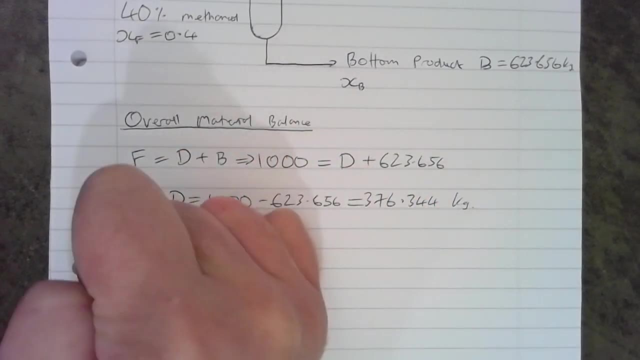 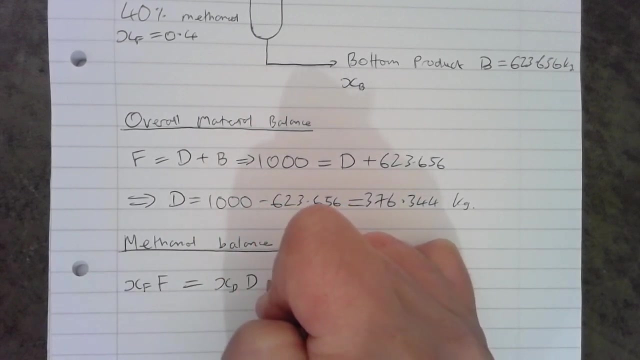 We can then do a component balance on the methanol. so methanol balance- and again we know what goes in must come out. so methanol in is XF times F equals XD times D plus XB times B. We know that the mass fraction of methanol going in is 0.4 times 1000 kilograms going. 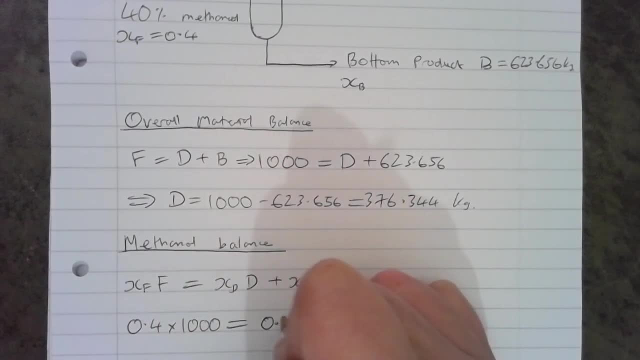 in equals the 0.98 mass fraction of methanol in the distillate times, the 376.344 that we just calculated, plus XB times 646.344 kilograms, That's 0.4.. 0.4.. 0.4.. 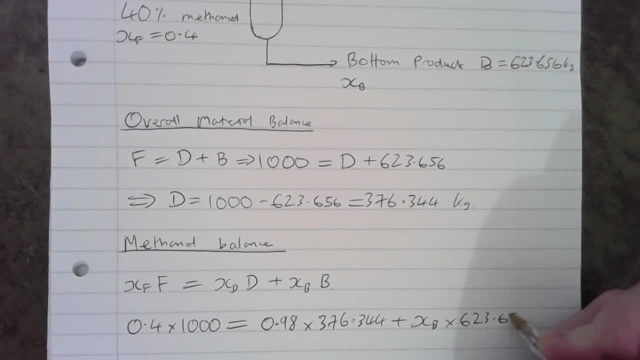 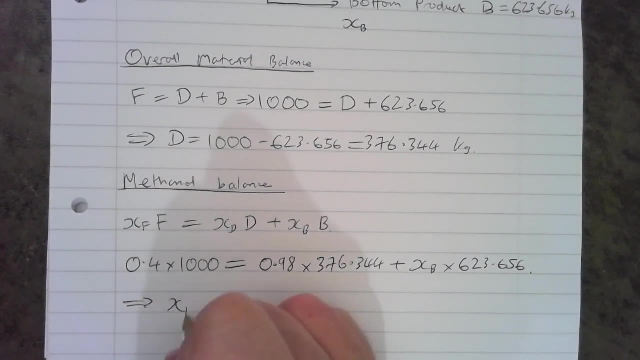 0.4.. 0.4.. 623.656.. Now, if we rearrange that we have, XB equals 0.4 times 1000 minus 0.98 times 376.344, all divided by 6..